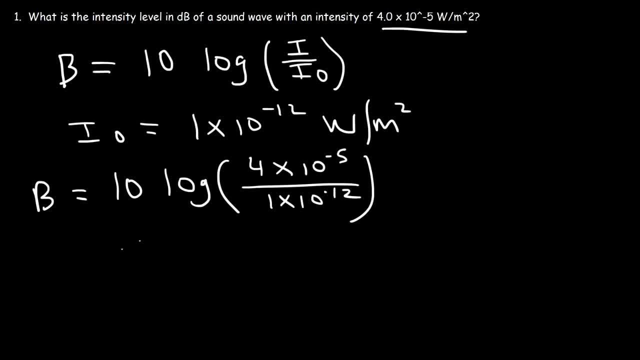 That's 7.6 multiplied by 10.. So the sound level is 76 decibels, And so that's a simple way to calculate the sound level, given the intensity of a sound wave. Now, what if we're given a sound level in decibels and we'll need to calculate the intensity? 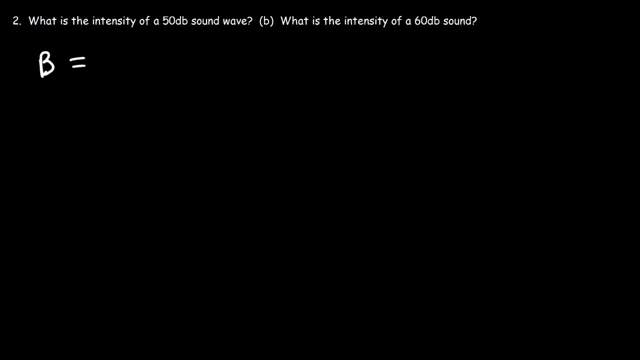 Well, we'll need to rearrange the formula. So let's start with this equation. Our goal is to solve for that variable, So the first thing we need to do is divide both sides by 10.. So the sound level divided by 10.. 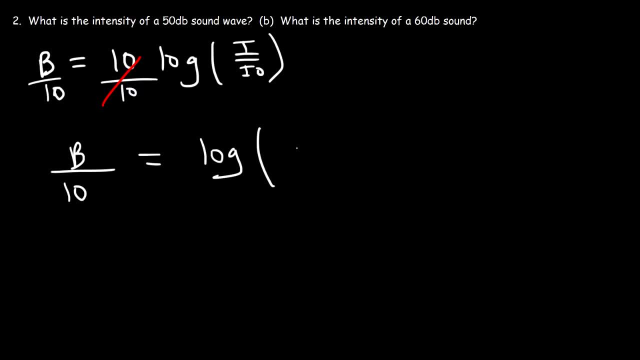 That's going to equal log of the intensity divided by the threshold of hearing. Now the next thing that we need to do is convert the logarithmic equation Into an exponential equation, And so let me give you an example of that. Let's say, if we have log base A of B is equal to C. 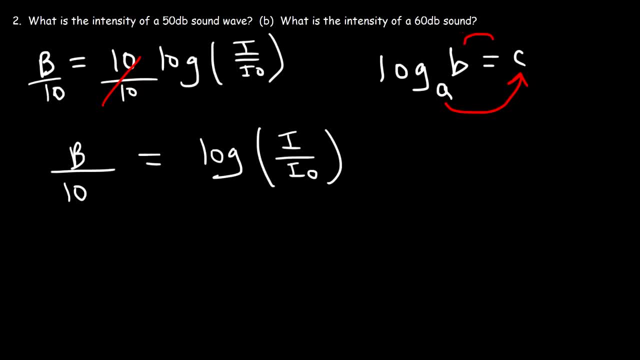 It turns out that A raised to the C is equal to B, So the base of log is base 10.. So 10 raised to B over 10 is equal to what's inside. So the stuff inside I over the threshold of hearing is going to be equal to 10 raised to the sound level. 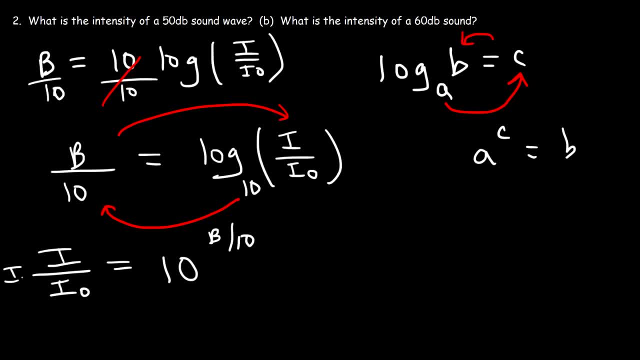 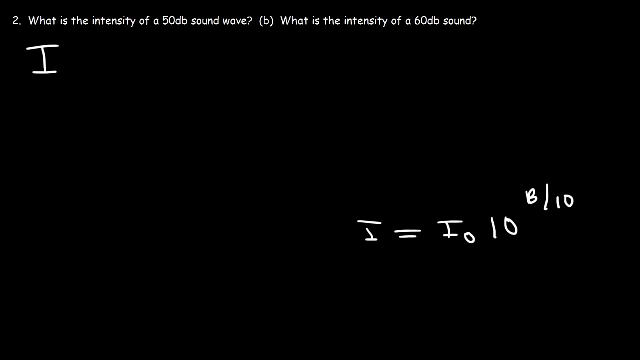 divided by 10.. Now the last thing we need to do is multiply both sides by. I naught So the intensity is the threshold of hearing times, 10 raised to the sound level, divided by 10.. So now we can get the answer. 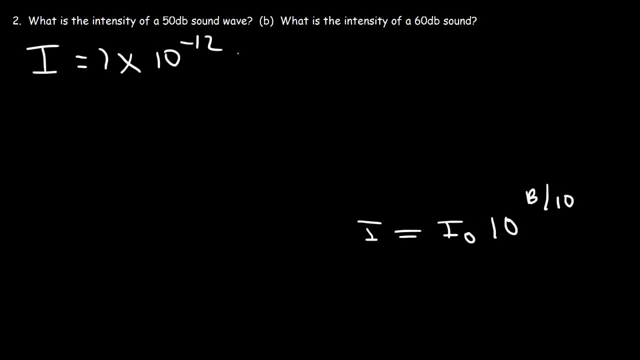 So it's going to be 1 times 10 to the minus 12, multiplied by 10, raised to the 50, divided by 10.. So 50 over 10 is 5.. So it's 10 to the 5, multiplied by 1 times 10 to the minus 12.. 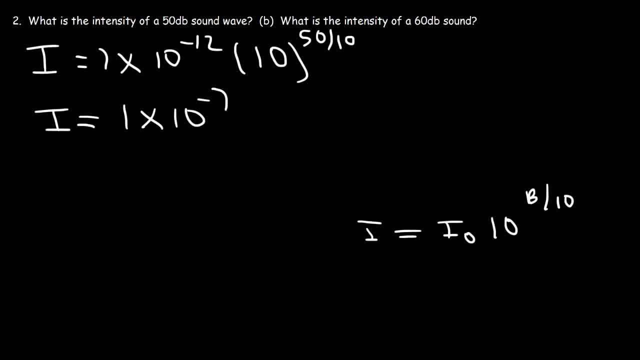 So the intensity is going to be 1 times 10 to the minus 7 watts per second. So that's going to be 1 times 10 to the minus 12.. So that's going to be 1 times 10 to the minus 7 watts per square meter. 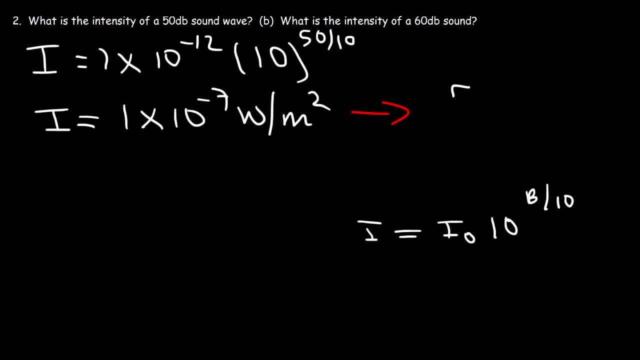 So that corresponds to a sound level of 50 decibels. Now, what about a sound level of 60 decibels? So it's going to be 1 times 10 to the minus 12 times 10, but 60 over 10.. 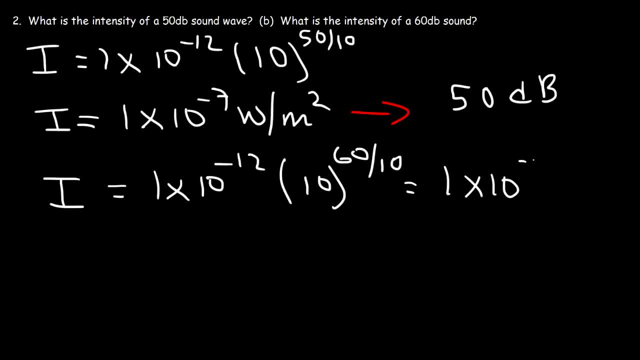 So the intensity is going to be 1 times 10 to the minus 12, multiplied by 10 raised to the sound level, divided by 10 raised to the minus 6 watts per second, So that corresponds to a sound level of 60 decibels. 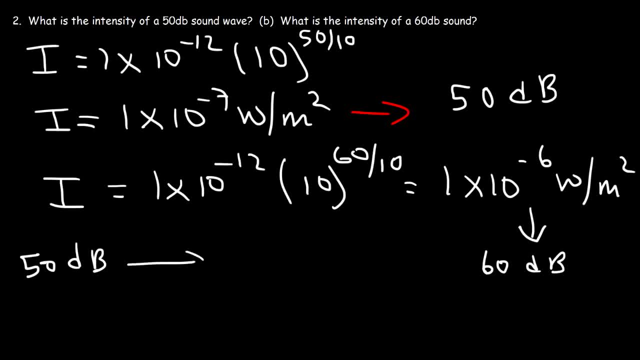 So notice when the sound level increased by 10 units. So when we add 10 decibels to go from 50 to 60 decibels, the intensity changed from 10 to the minus 6, actually 10 to the minus 7, to 10 to the minus 7.. 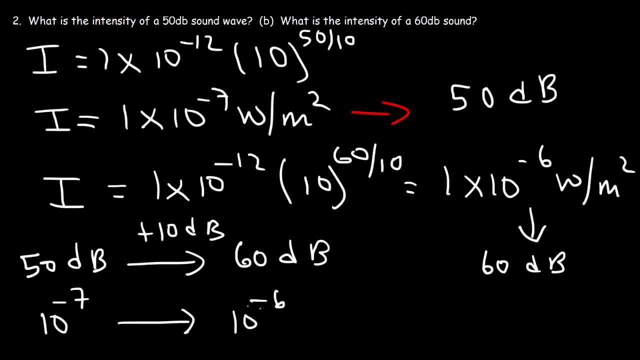 So that's going to be 1 times 10 to the minus 6 watts. So that's going to be 1 times 10 to the minus 6 watts. So that's going to be 1 times 10 to the minus 6.. 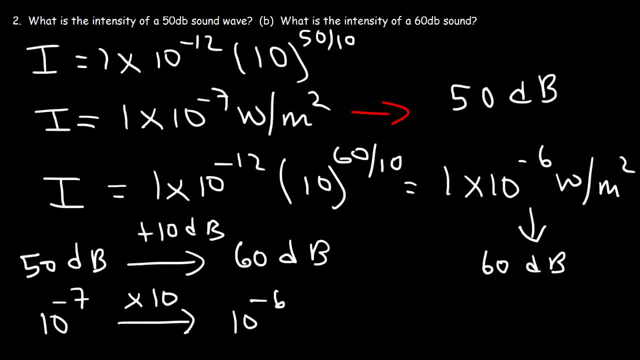 So it was increased by a factor of 10.. So notice that an addition of 10 decibel units increase the intensity by a multiplication of 10.. Make sure you understand that every time the decibel factor, or the sound level, increases by 10 decibels, the intensity gets multiplied by 10.. 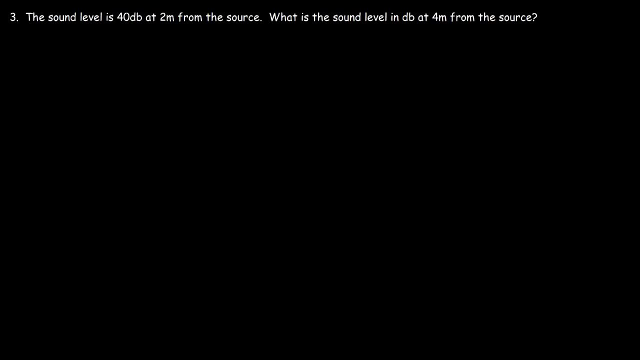 It's 10 times higher than what it was before. Let's move on to number 3.. The sound level is 40 decibels at 2 meters from the source. What is the sound level in decibels at 4 meters from the source? 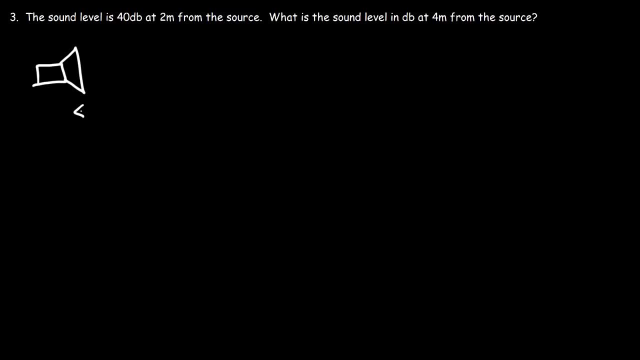 So let's say, if we have a speaker- So at a distance of 2 meters it's 40 decibels- What's going to happen to the sound level if we double the distance? What's the new sound level going to be? 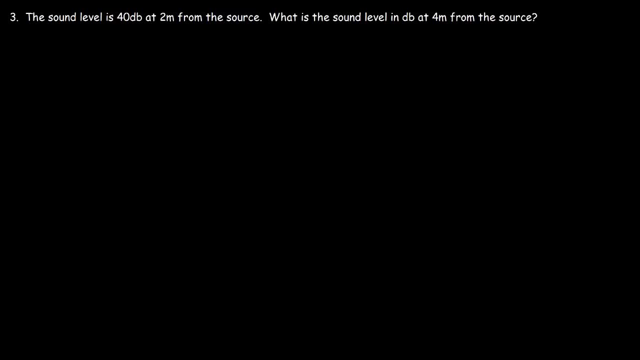 10.. Well, let's come up with an equation that's going to help us to get that answer. So we know that intensity is- I naught- times 10, raised to B over 10.. And also, intensity is power divided by area. 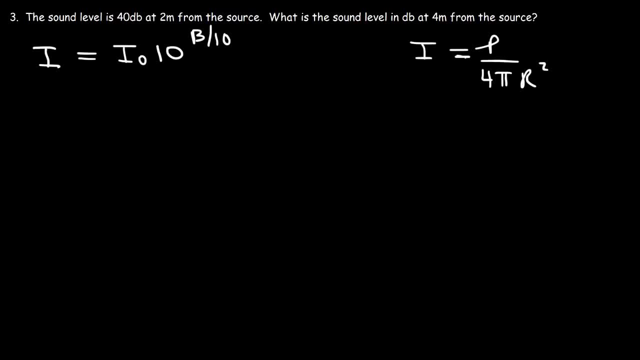 And this is the surface area of a sphere. So we need to connect the distance, which is basically r, with the decibel levels, which is B or beta. How can we connect these two together? Well, first let's find the ratio of intensities. 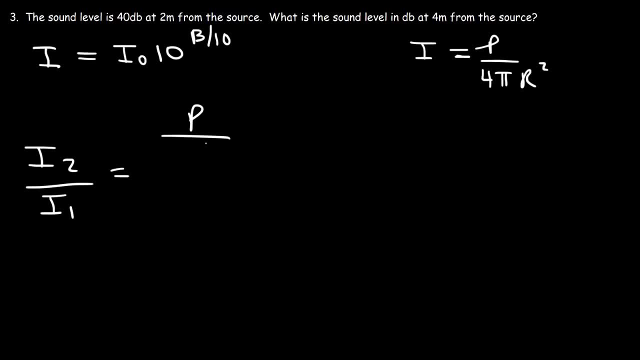 So I2 is going to be P over 4 pi r2 squared And I1 is going to be P over 4 pi r1 squared. Okay, So since we're dealing with the same source, it's going to emit the same power. 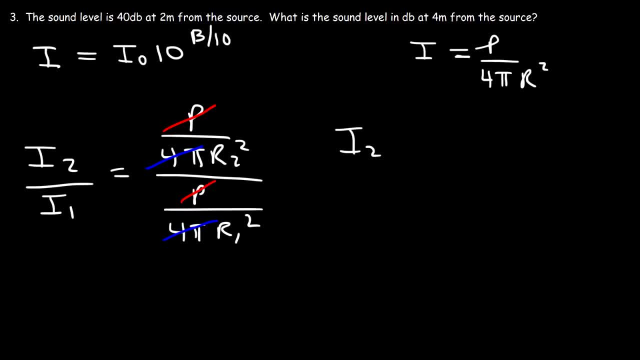 And 4 pi is the same. So I2 divided by I1 is going to be 1 over r2 squared divided by 1 over r1 squared. Now I'm going to multiply the top and the bottom by r1 squared. times r2 squared. 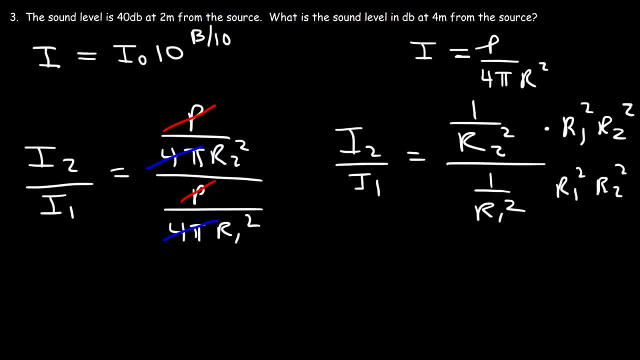 Whatever you do to the top, you must also do to the bottom, So that the value of the fraction is equal to r2 squared And the value of the fraction remains the same. So these will cancel. So r1 squared is going to be on the top and r2 squared is going to be on the bottom. 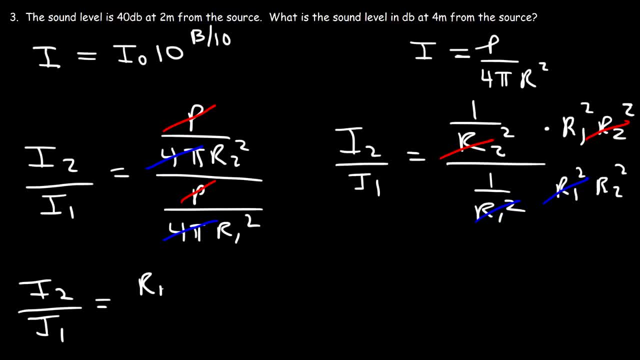 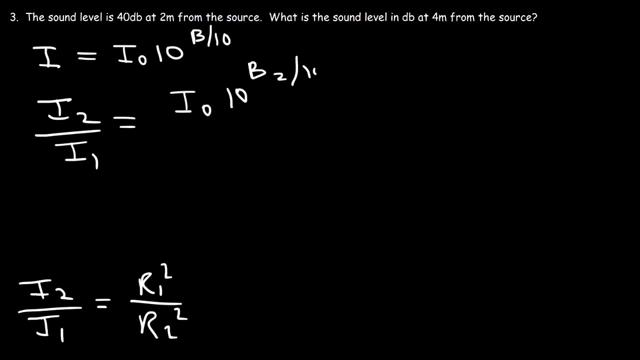 So I2 over I1 is going to be r1 squared divided by r2 squared. Now let's focus on this equation. So once again, let's take the ratio of two intensities. So I2 is going to be I0 times 10, beta 2 over 10.. 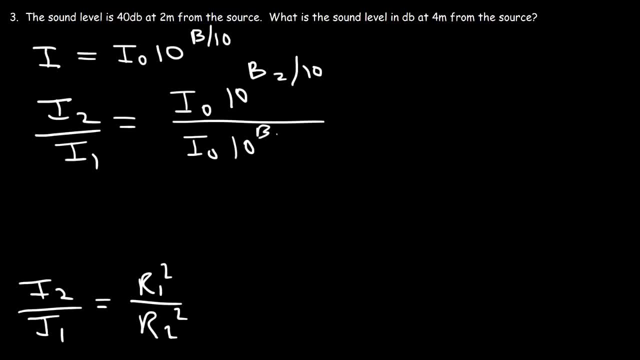 And I1 is going to be I0 times 10, beta 1 over 10.. So we can cancel these two. Now, when you're dividing using a common base, you need to subtract the exponents. For example, x to the 7 divided by x to the 3rd is x to the 7 over 10 squared. 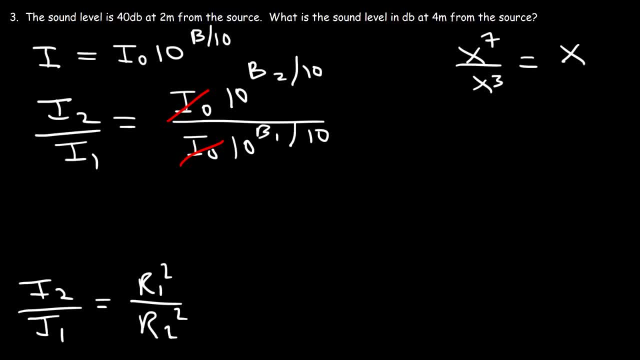 So I1 is going to be I0 times 10, beta 2 over 10.. And I1 is going to be I0 times 10, beta 1 over 10.. So we can cancel these two. So this is going to be b2 over 10 minus b1 over 10.. 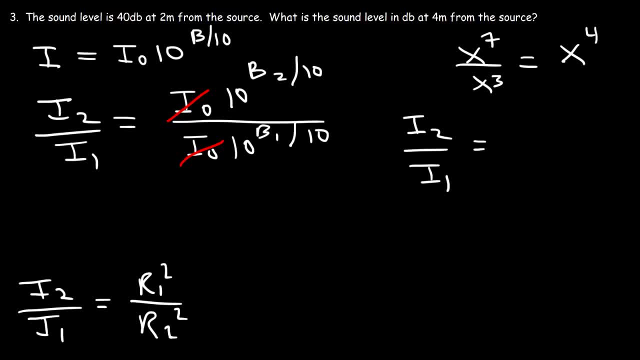 So we can say that I2 over I1 is equal to 10, b2 over 10 minus b1 over 10, which, because they have the same denominator, we could simply say it's just b2 minus b1 over 10.. 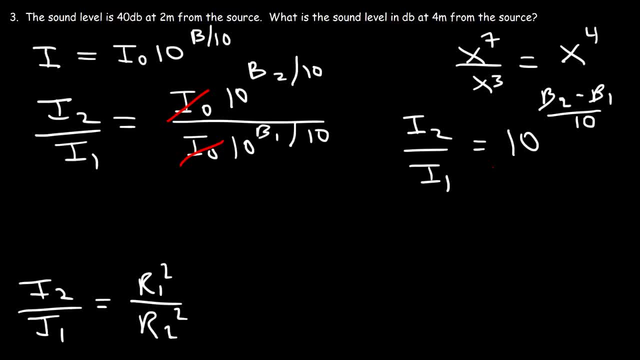 So now we could set This term equal to that, because they both equal I2 over I1.. So R1 squared over R2 squared is equal to 10, b2 minus b1 over 10.. So now what we need to do is take the log of both sides. 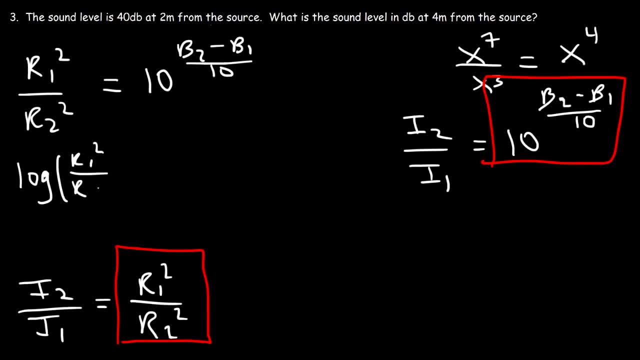 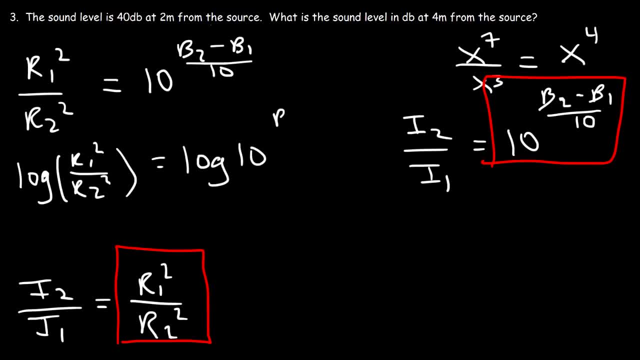 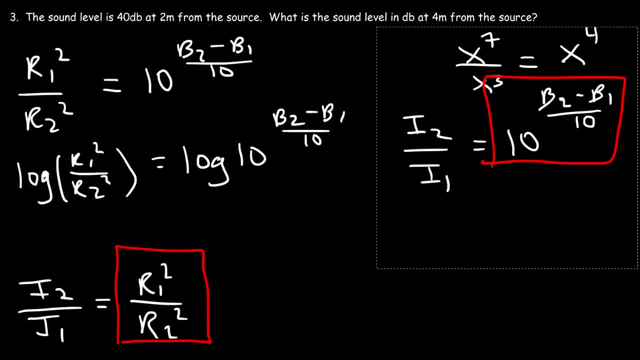 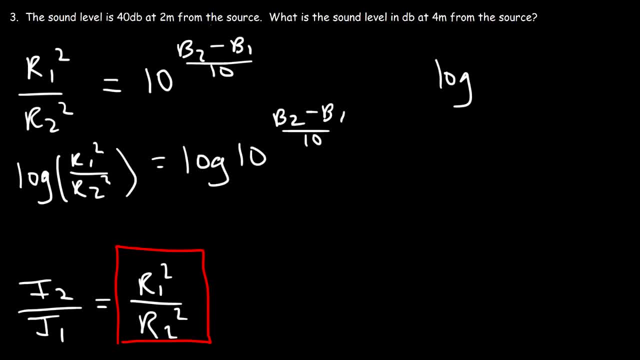 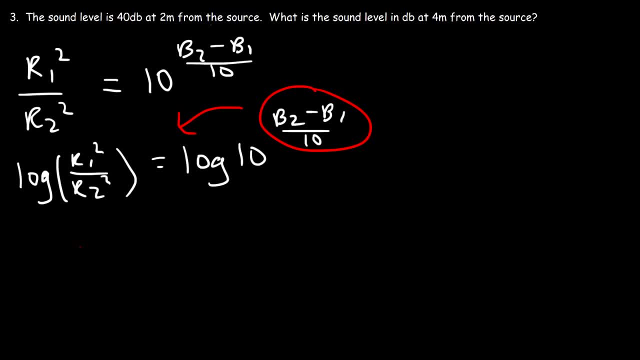 So therefore we could take this term, move it here. So on the left we have log r1 over r2, and I'm just going to put the square on the outside- which is equivalently equal to that, and this is equal to b2 minus b1 over 10 times log 10.. 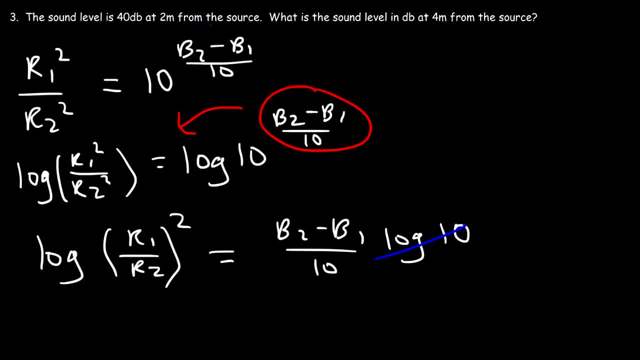 Log 10 is 1, so we don't have to worry about this thing and I'm going to move this 2 to the front. So now I have 2 log r1 divided by r2, and that's equal to b2 minus b1 over 10.. 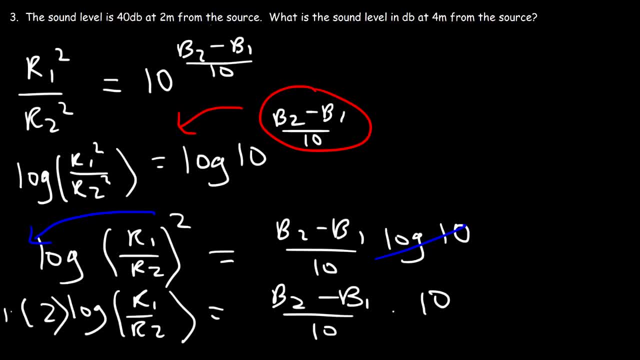 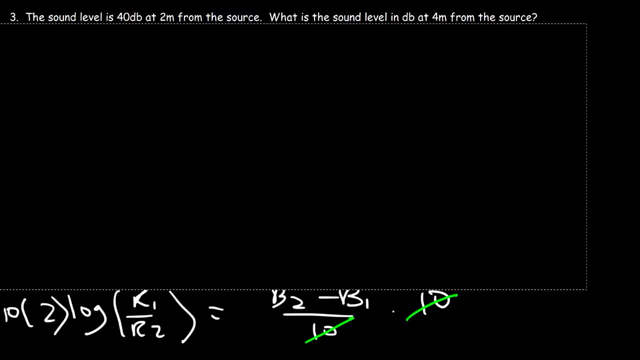 So now I'm going to multiply both sides by 10.. So on this side all I have is b2 minus b1. And on the left side I have 10 times 2, which is 20, times log r1 divided by r2..